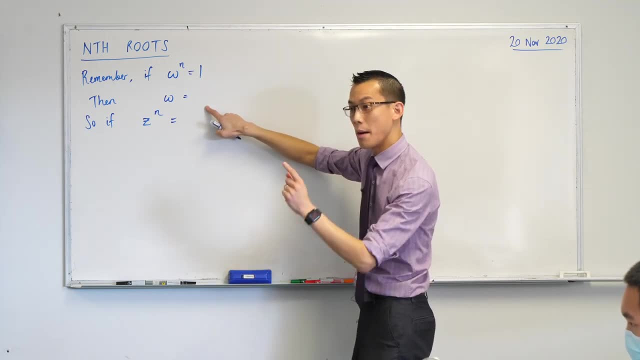 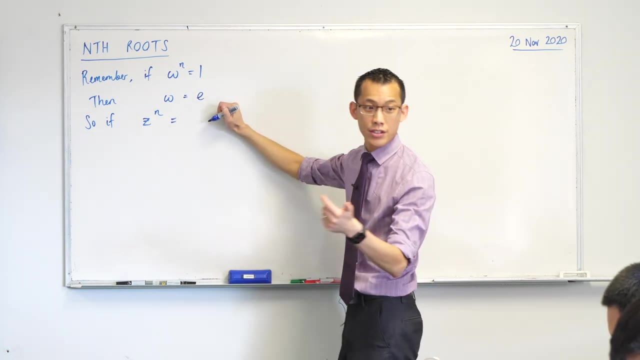 So, rather than just write one which is in rectangular form, I'm going to write it in exponential form. It's going to start e to the power of what i times 0. The argument is 0,, isn't it? So you get that. 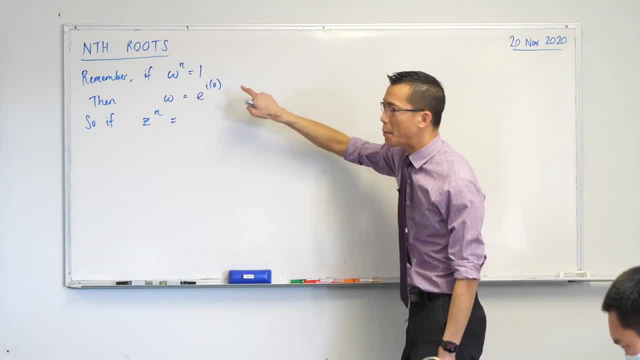 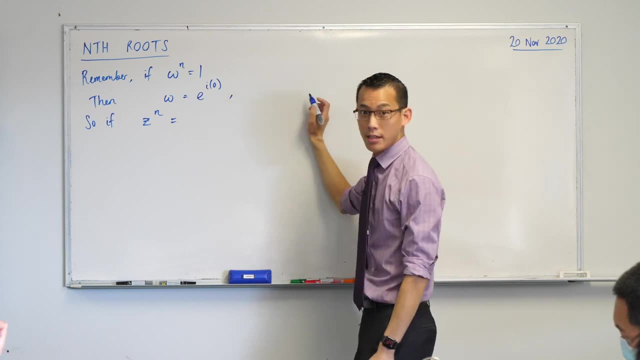 And then what we did was we had a look at cube roots. so I would then go: oh, I'm expecting two more solutions, Polynomial of degree 3, three complex solutions. So then I started to list here right Now, if I'm saying to you: oh, I don't know what particular root, 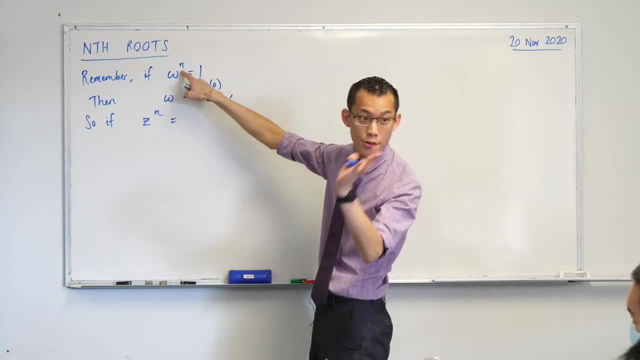 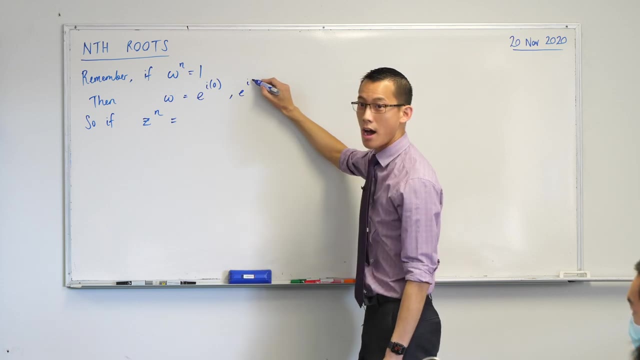 Of unity we're after could be six or seven or eight or a hundred or something like that. I would have to extend this, however long, right? So I would say, the next one would come from e to the, i to pi, And then I would go to the next one. 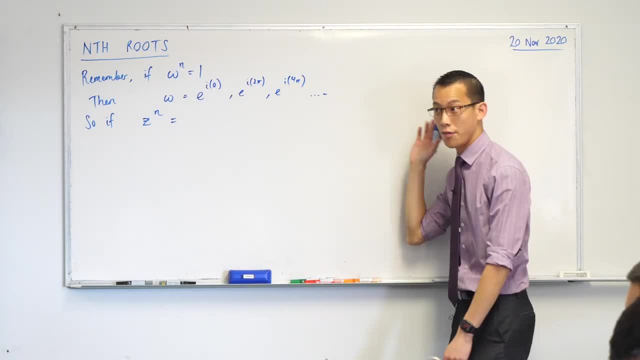 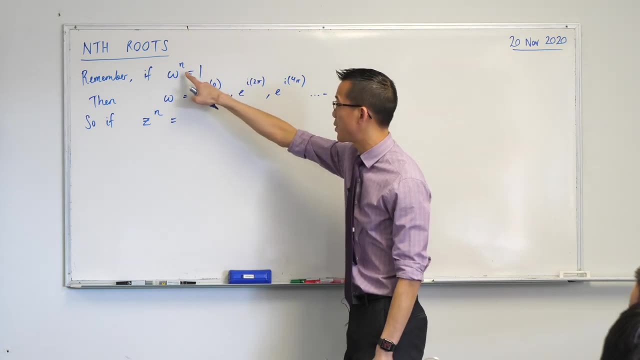 And then I would just keep going until I've got n of them right. Does that ring a bell? Now, here's the thing I would have to say. this is w to the n, but I want to raise both powers to 1 over n. 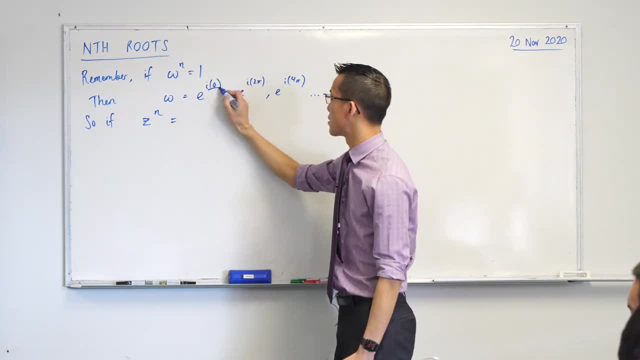 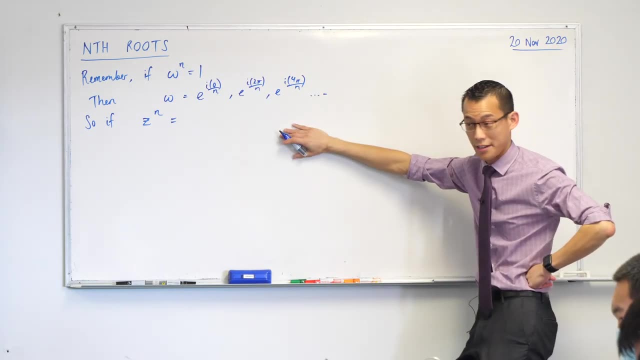 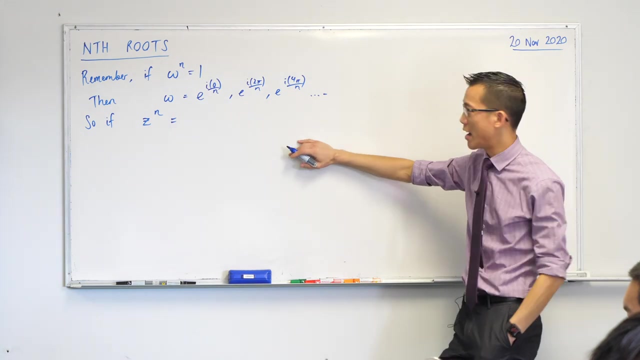 That's the same effect as taking the nth root. So I would do this: I would divide this by n, this by n, this by n, and then off I go. These are the nth roots of unity. So what we're going to do is then take that idea and say: well, what happens if we have any complex number? right? 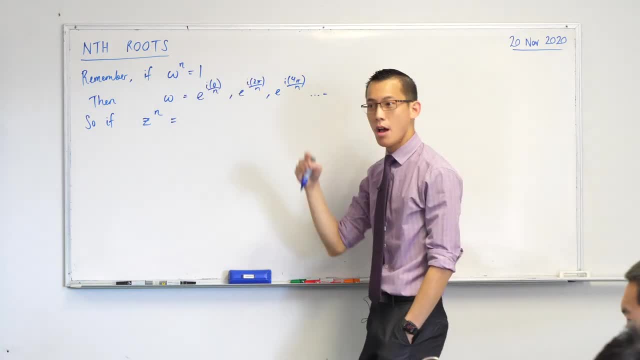 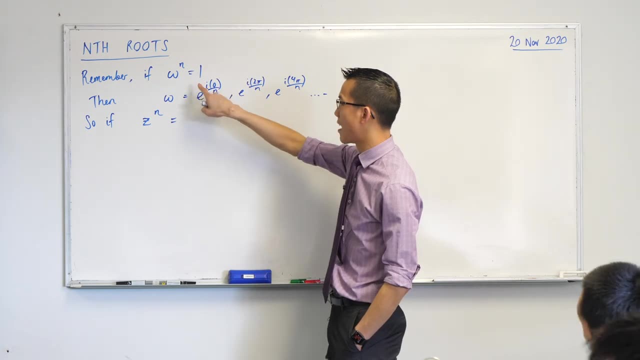 Not just one unity, which is sort of special. but what if we had some arbitrary complex number? So the first thing to say is, if you have some arbitrary complex number, it might not be one unit away. It might not be one unit away. 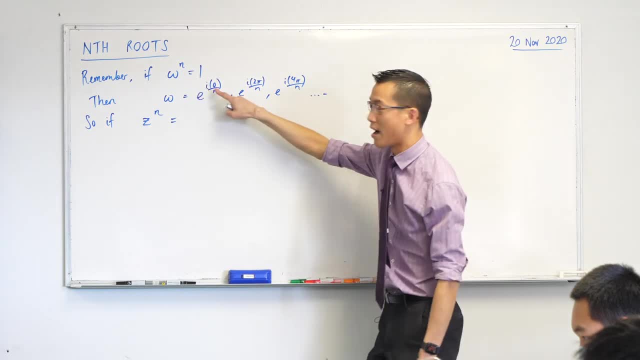 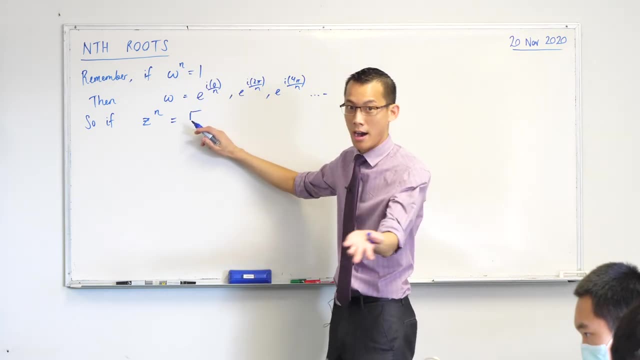 It might not be one unit away, It might not have a modulus of 1.. So instead of just saying e to the i 0, I'd have to say r to indicate my modulus. It could be anything right. I mean, it might be 1, but it could be a half. 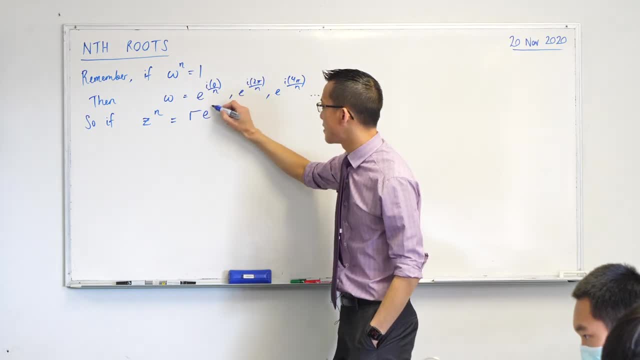 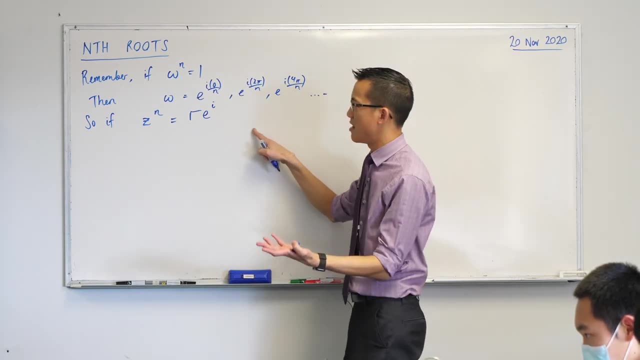 It could be root 3, anything you want. I've got my e to the i up here, which is always part of exponential form, But if I'm letting this be any complex number then it could have any angle. It might not just start with 0. 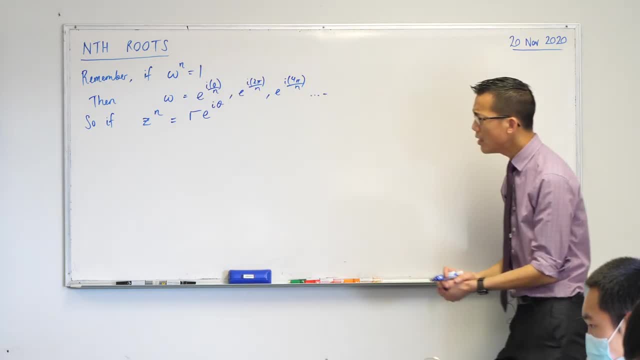 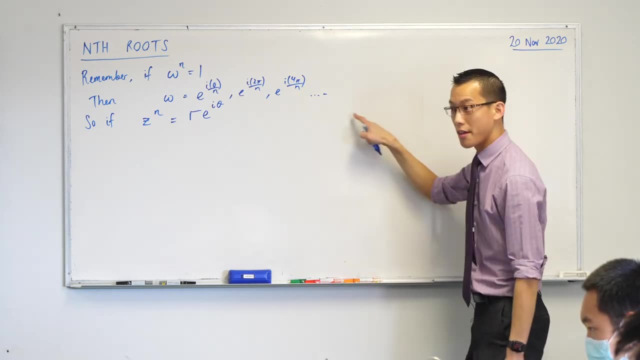 So I'm going to indicate that with a theta. OK, So if we have this being true, Then I can also say, just like in the previous line, I've got all of the other versions of that complex number right With non-principal arguments. 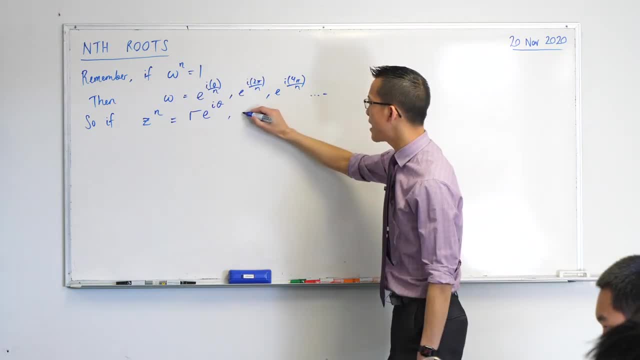 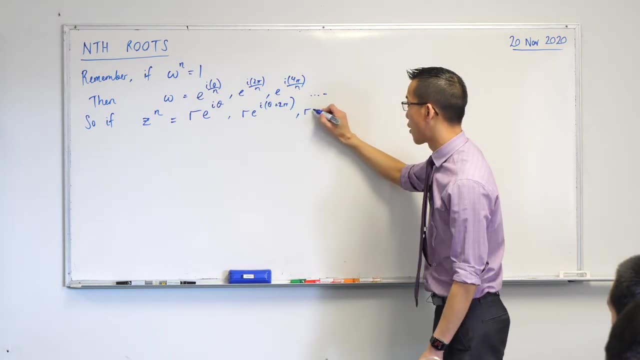 Do you remember that? So let's go ahead and write them in here. I can say it's r? e to the i? theta plus 2 pi. That would be the next one around, And then I could go r? e to the i? theta plus 4 pi. 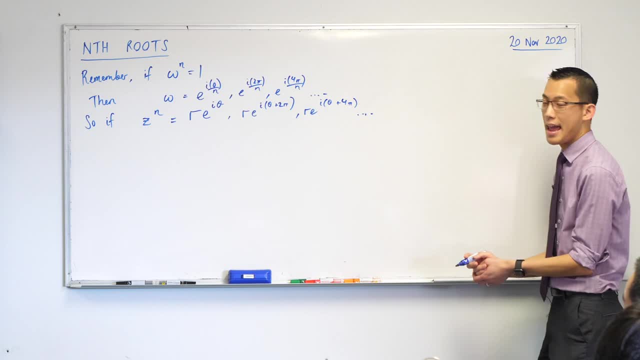 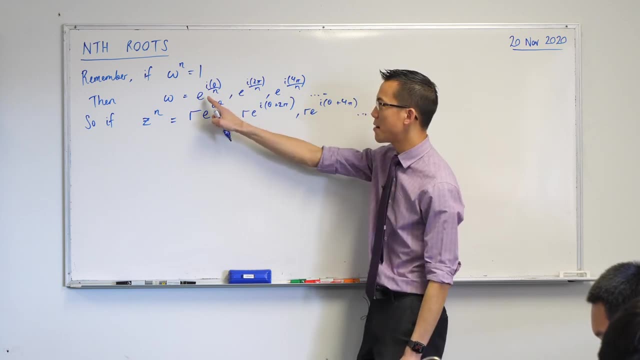 That would be the next one around after that, And I could keep going and I would have n of them, And the process is going to be the same. If I want to take the nth roots of these numbers, then it's the same as raising both sides to the power of 1 over n. 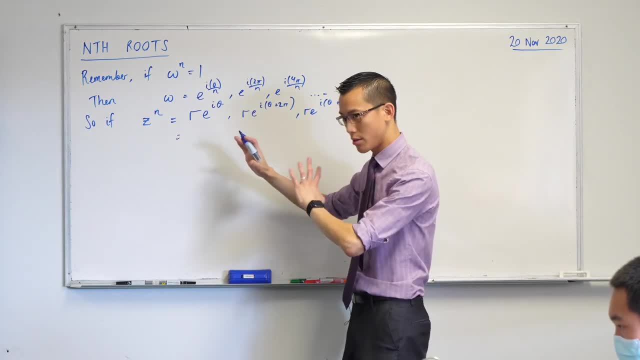 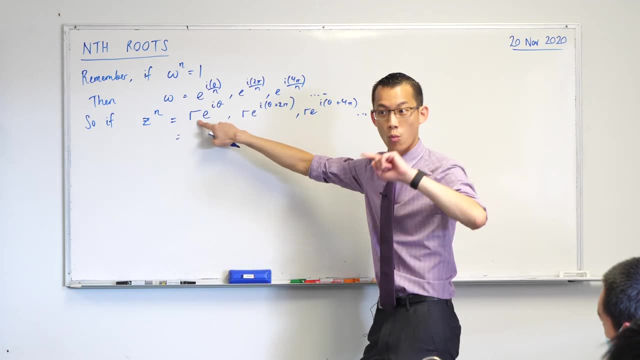 Is that OK? So let's go ahead and write that in, And then we can notice some patterns here. When you raise a number like r, the modules right A real number to the power of 1 over n. That's the same as taking the nth root of that number. 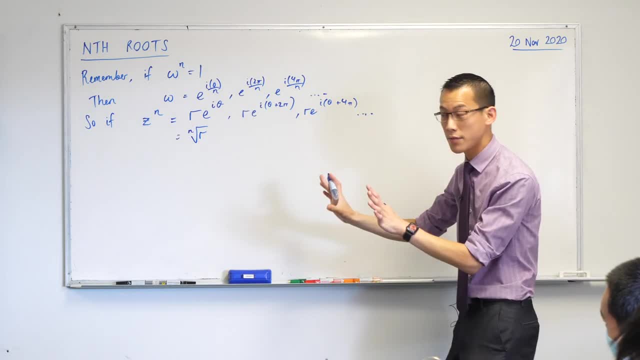 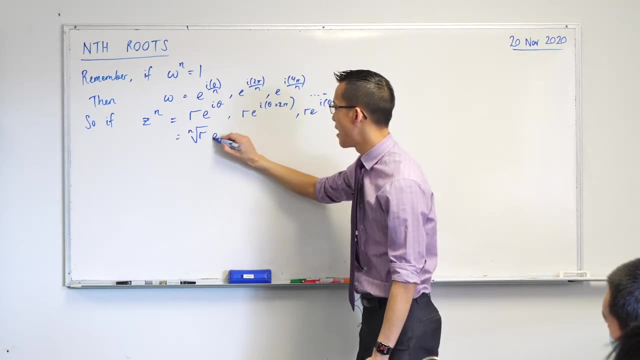 Do you agree? OK, so we can just do that with a real number. That's fine, But then, when we come to these guys, we have to deal with these, These exponents, these indices that we have. So I'm going to raise e to the power of i theta on n. 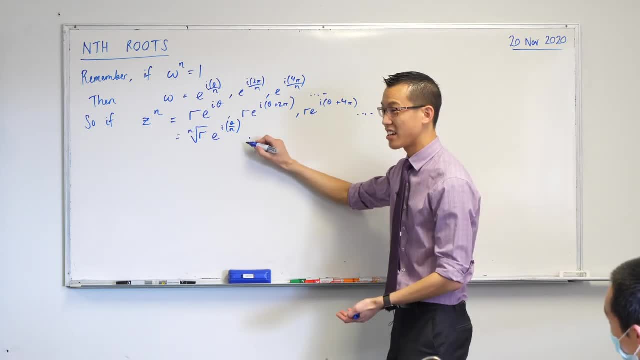 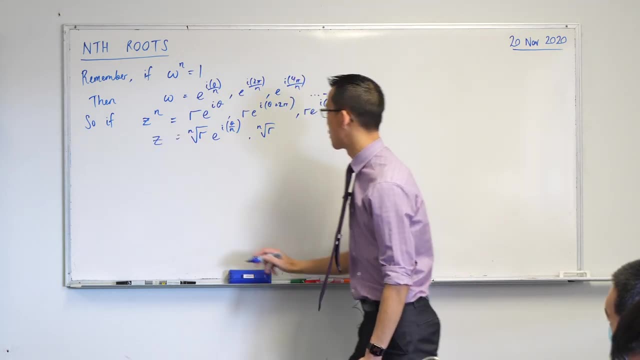 Do you agree with that? That's me dividing by n in the index, And then I just kind of keep going right. I've still got the nth root of r as my modulus for my nth root here, And then I'm going to divide this by n as well. 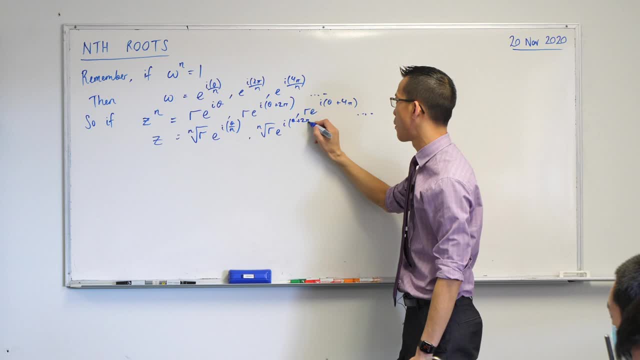 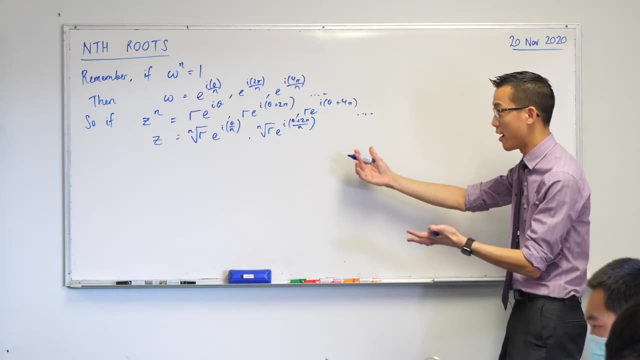 So I'm going to go i and then theta plus 2 pi. That's divided by n And it starts to get a bit. It's almost kind of Like I'm on autopilot here, because I don't have to think too hard. 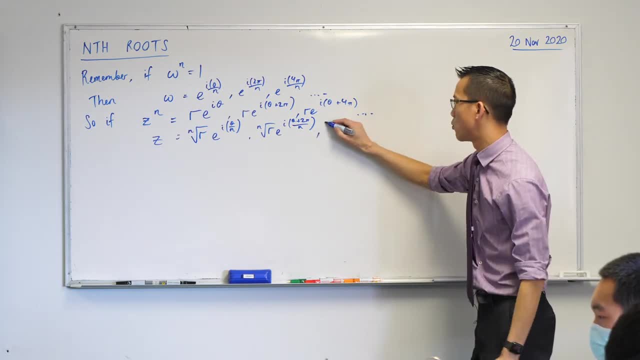 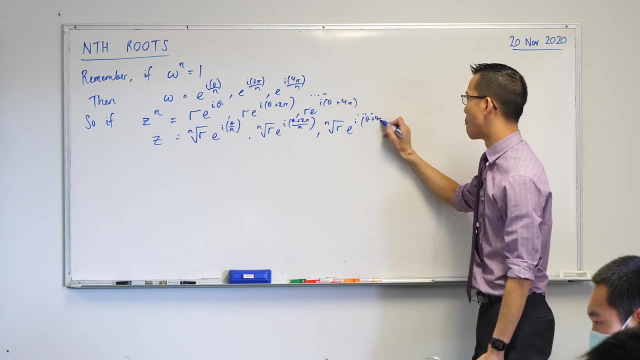 because exponential form is built to do this right. So I'll just do one more for good measure, to sort of establish the pattern. So I've got e to the i theta plus 4 pi on n. There we go And then continue going until you have n of these. 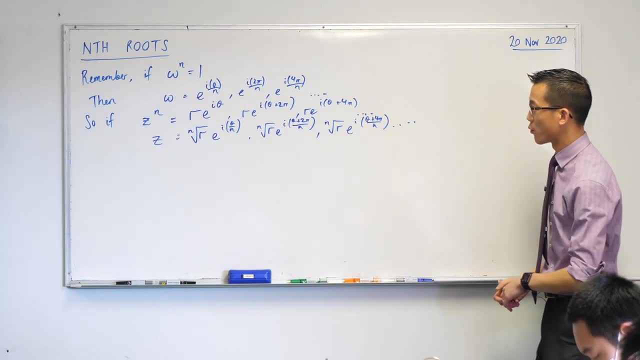 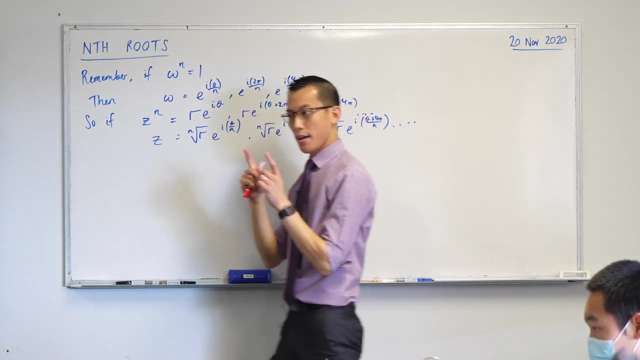 Now I want to highlight two important differences, which are really the key to these nth roots of any complex number, versus our nth roots of unity. OK, My nth roots of unity line, our second line here. right, We can say that all of the roots of unity. 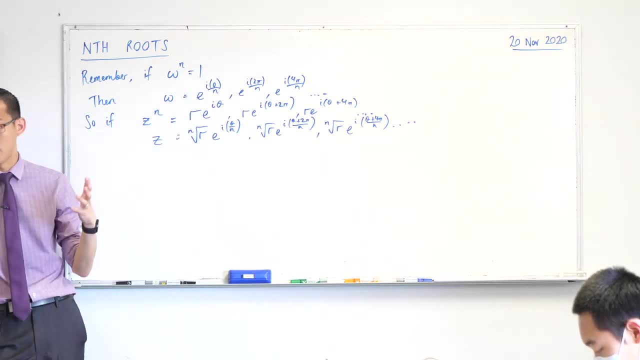 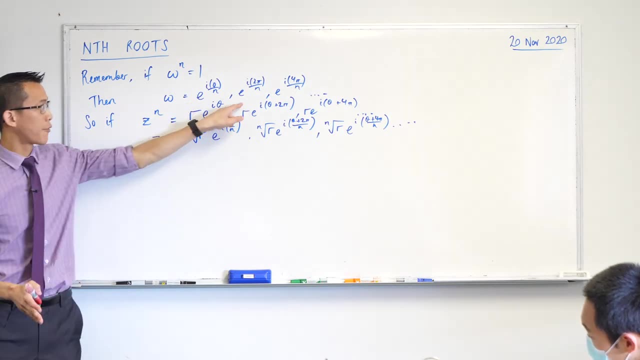 no matter what root of unity you're after- second root of unity, third, fourth, 100, they all lie in the circumference of the same circle. right Which circle is that? It's the unit circle, because what's implied out the front here is a 1.. 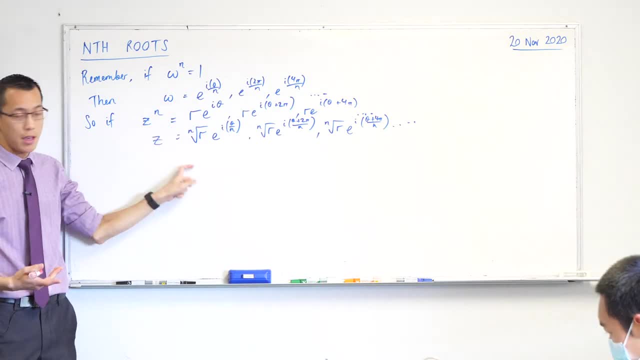 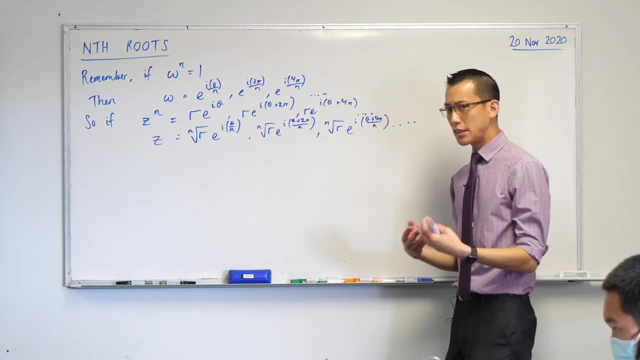 So the modulus is 1 for all of these nth roots. OK, These guys do not lie on the circumference of the unit circle, at least probably not if our modulus is not 1, right, But they still lie on the circumference of a circle, right? 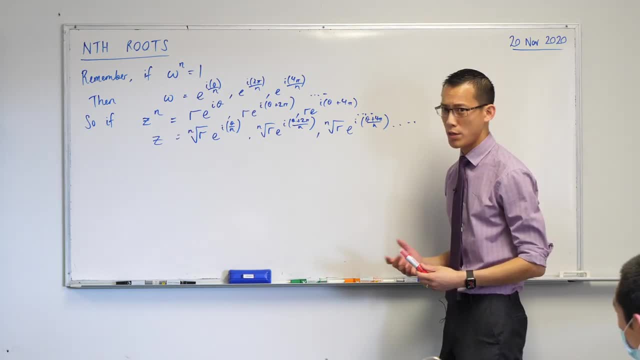 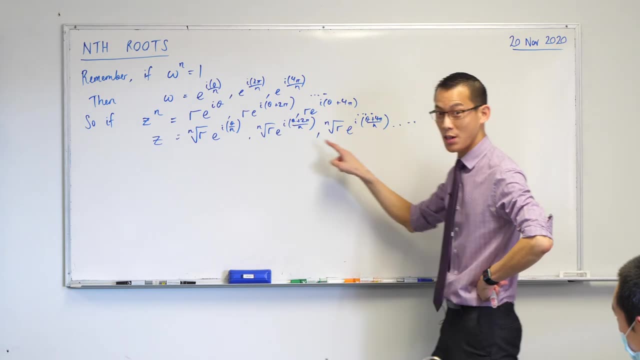 What can you tell me about that circle? Where's it's center? Have a think about this: All these complex numbers lie on the circumference of the circle which has the same center. Where's the center? It's still the origin, isn't it? 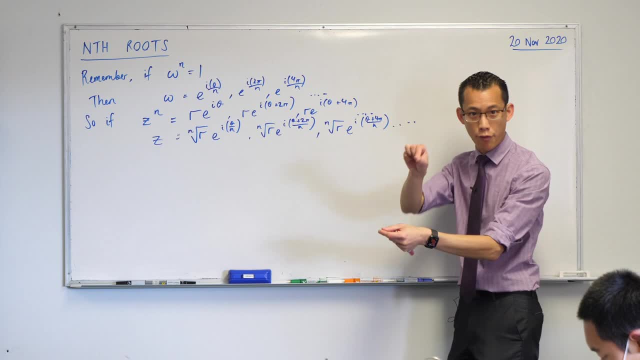 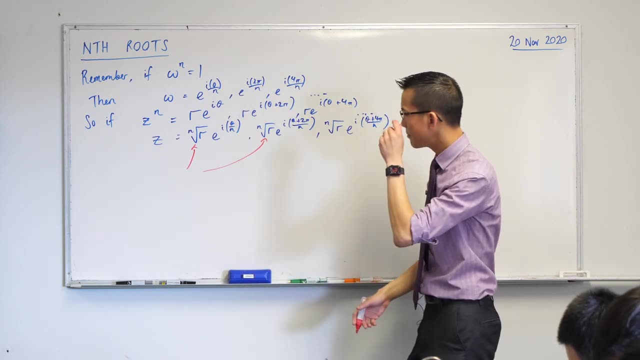 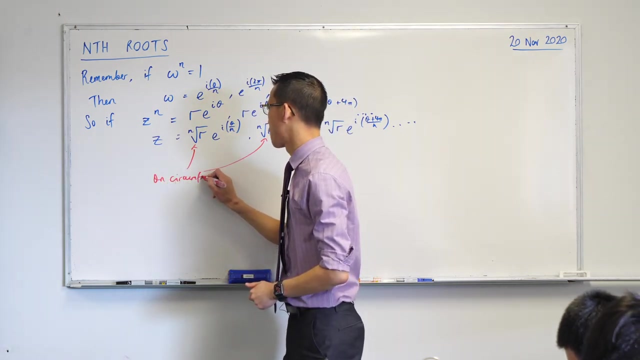 Because this modulus is always by definition measured from 0, right. So I'm going to note that down. I sort of get that from these moduli over here that these are still on the circumference of a circle. It's just a circle on circumference of. 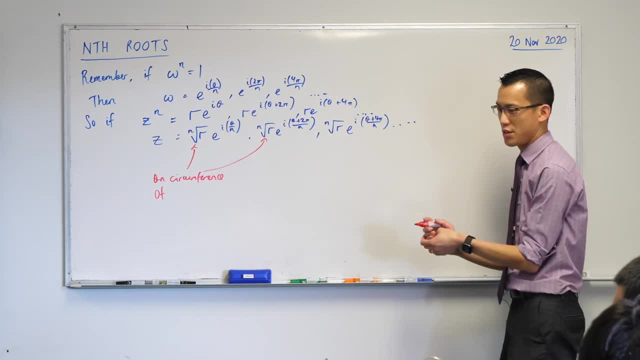 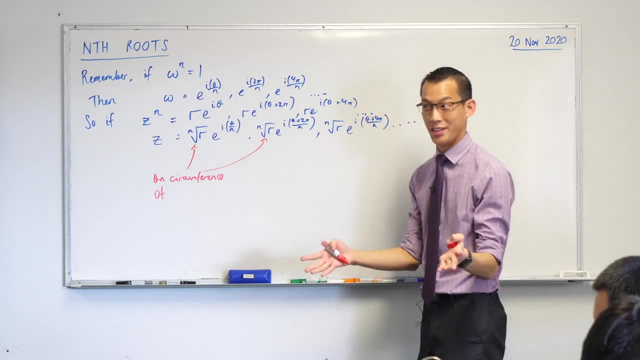 Now I want to write the equation of this circle, So I'm going to actually lean forward with a slight spoiler into next week's. If I want to talk about what the equation of a circle is, you don't have to write this down. 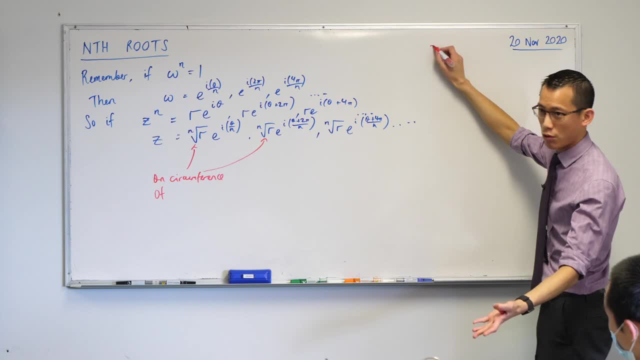 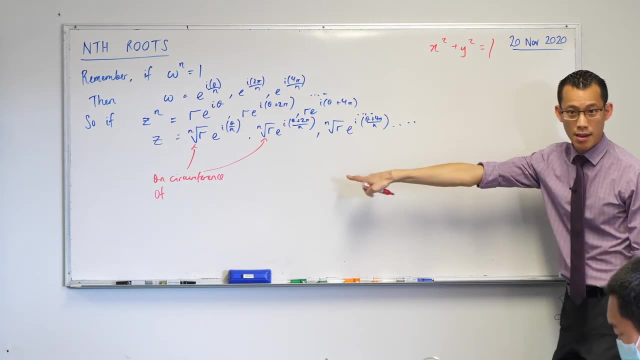 You would normally say in Cartesian terms. say, for example, the unit circle would be: x squared plus y squared equals 1. We recognize this. We've seen this before. OK, Now we could write it like this Here. but we have complex number sort of terminology to help us right. 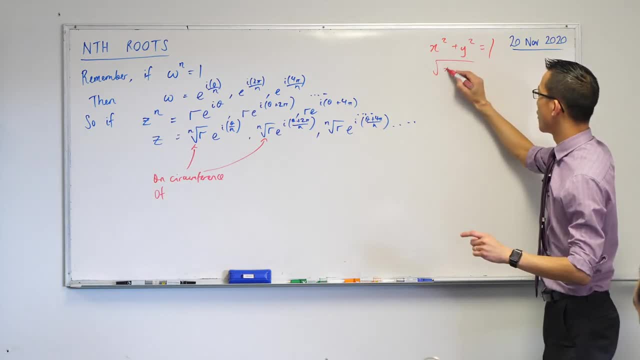 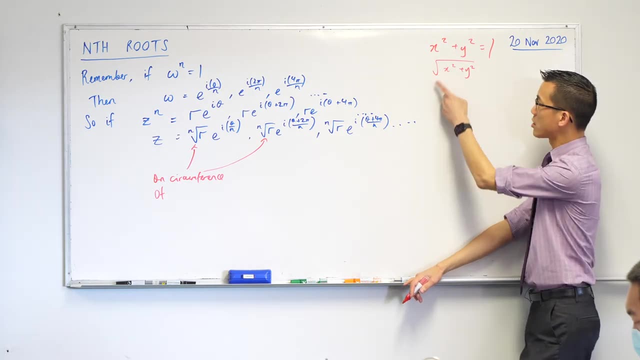 x squared plus y squared. I recognize this: The square root of x squared plus y squared. I have a very simple term that gives me this: if my complex number is x plus iy, What is the square root of x squared plus y squared in the context of complex numbers? 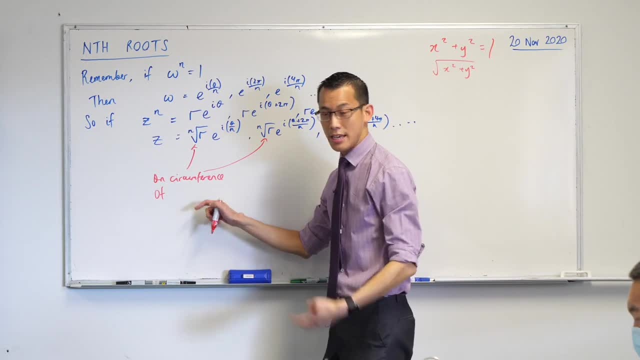 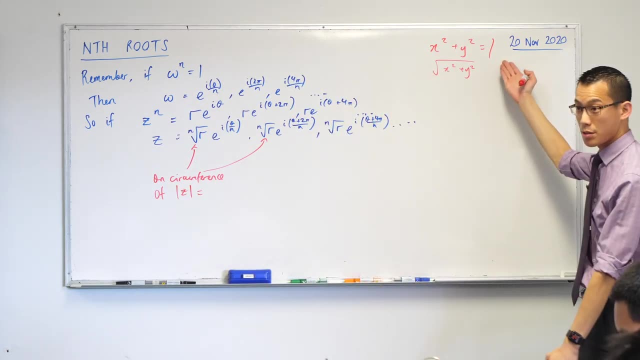 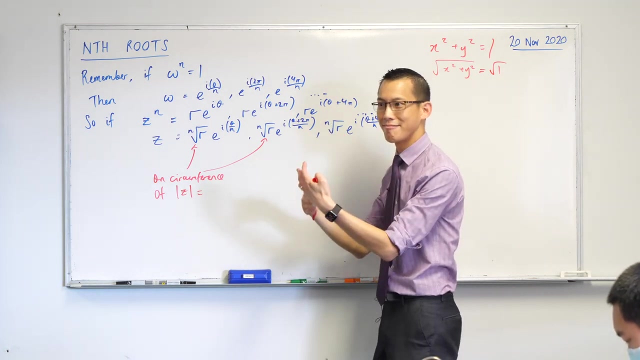 It's the modulus, isn't it? So I can say, a circle is all of the set of points where their modulus is some particular number, the radius. In this case it would be 1.. But in this case over here we just discovered, our radius is not just 1.. 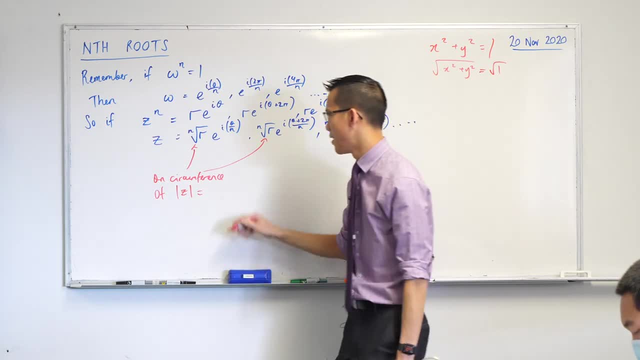 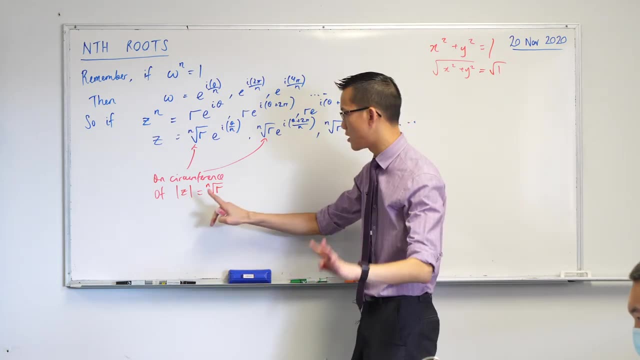 It'll be the nth root of r, whatever modulus. that was OK. So I'm going to write that in here. Still on a circle, still center at the origin, but its radius can change. That's the first thing. The second thing is we've got this spacing right. 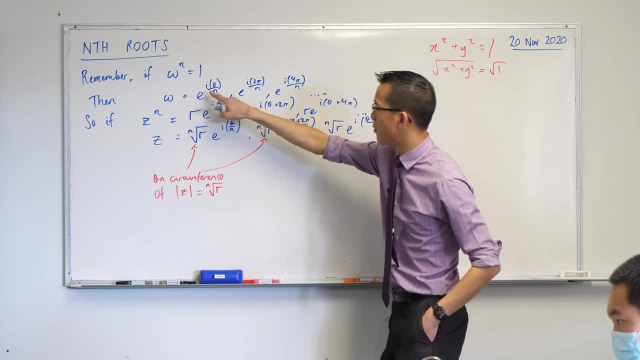 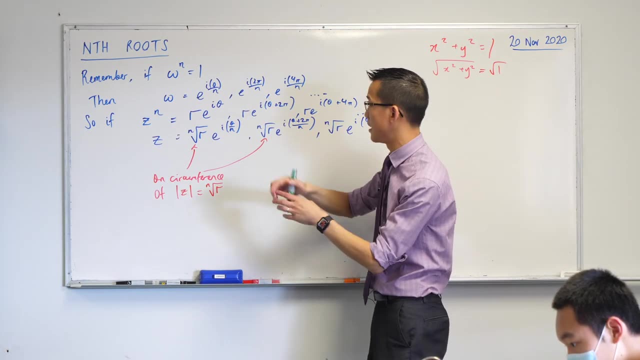 It's the same spacing that you saw here. from this solution to the next one. It's going to be 2pi on n difference, right? So, for example, when we looked at the cube roots of unity when we went from here to here, that example was 2pi on 3, right. 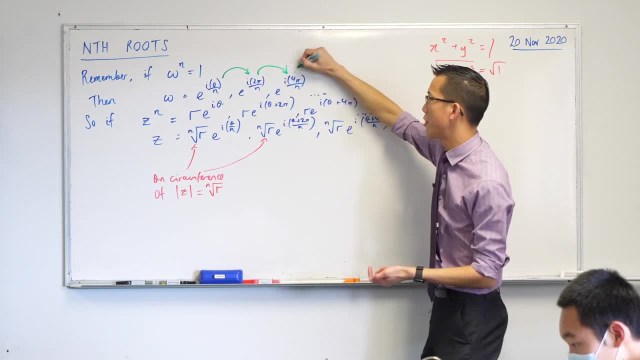 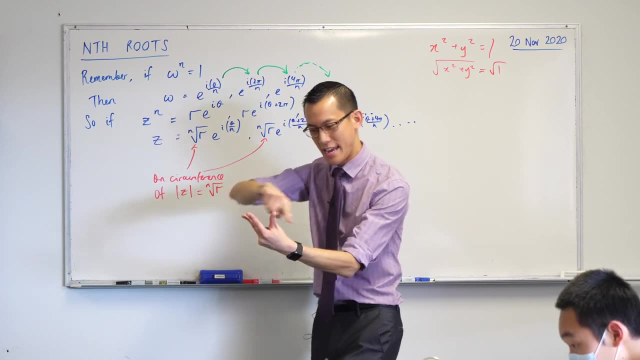 And then you went again another 2pi on 3.. And then if you went a third 2pi on 3, you would end up back at the start, right? Because 2pi on 3 plus 2pi on 3 plus 2pi on 3 is 2pi. 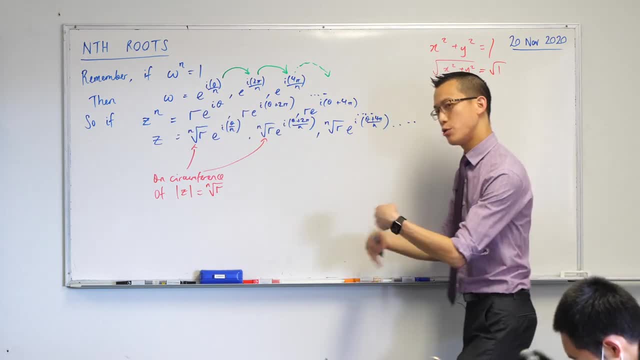 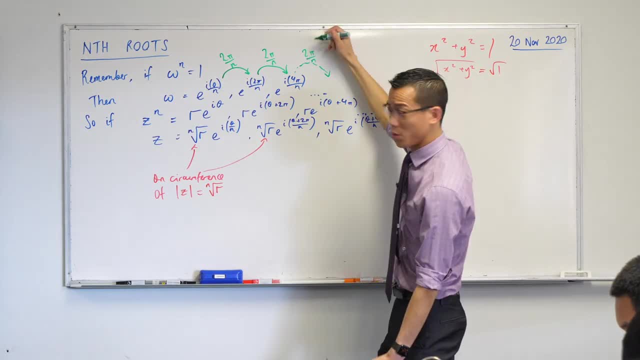 So there's 2pi on n where n can change right. 2pi on n that I'm going to call it a spacing right. We noticed this last time. You've got this equal spacing around the unit circle. 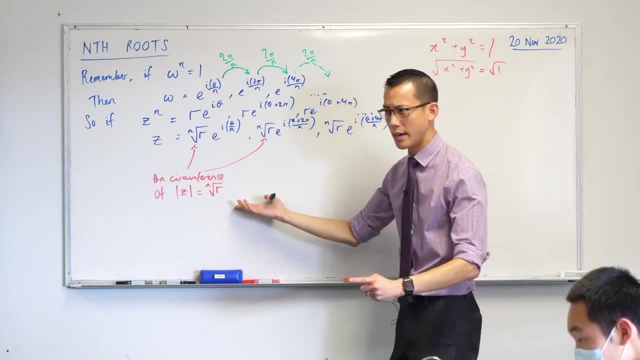 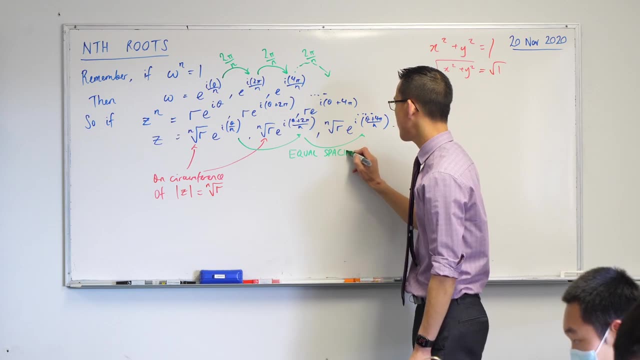 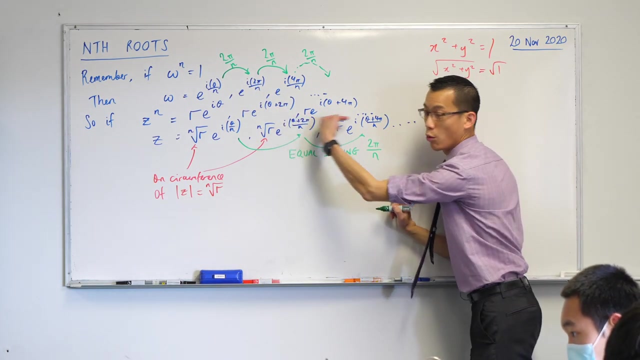 I still had this same equal spacing. It's just around a different circle, Is that OK? So you've still got this equal spacing. But even the spacing itself of the arguments is the same: 2pi on n all the way through. 2pi on n all the way through. 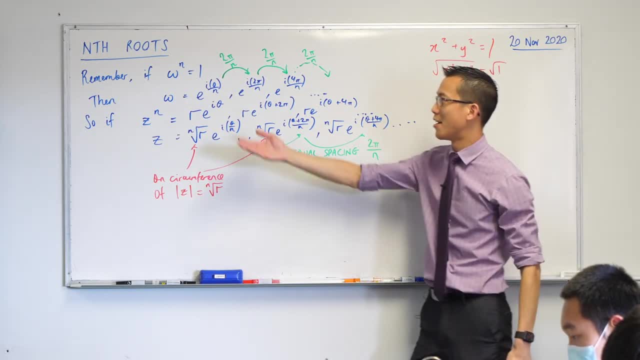 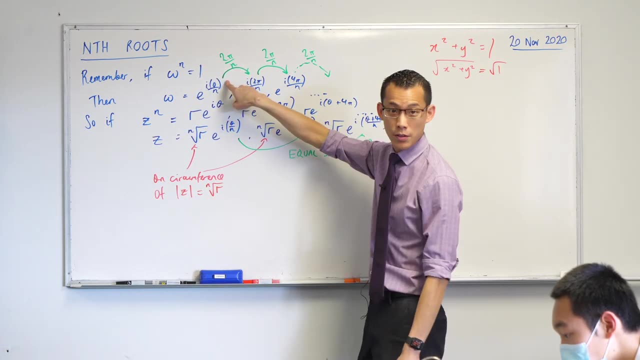 The only subtle distinction is because you don't have the nice neat fact that you know where the first root is. every time, for the roots of unity, The first root is always going to be 1.. Argument is 0.. Here your argument doesn't automatically start with 0. 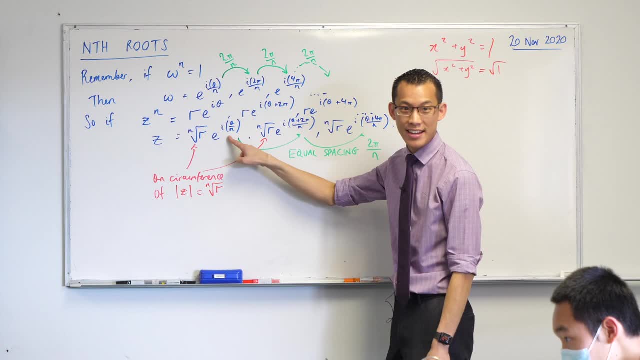 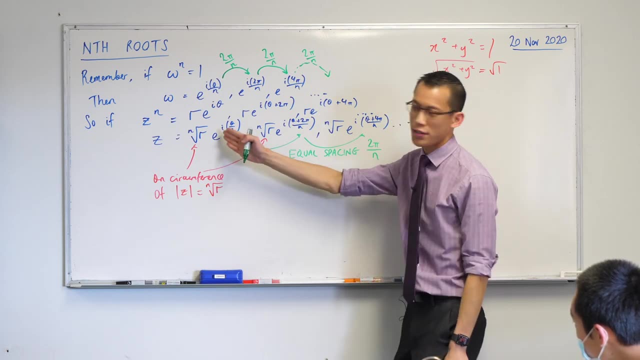 So, therefore, your first solution won't necessarily be at 1, right? So therefore, even though you still have the same equal spacing, you have to say: but your first solution doesn't start at 0. It can start at anywhere, depending on whatever your complex number was.